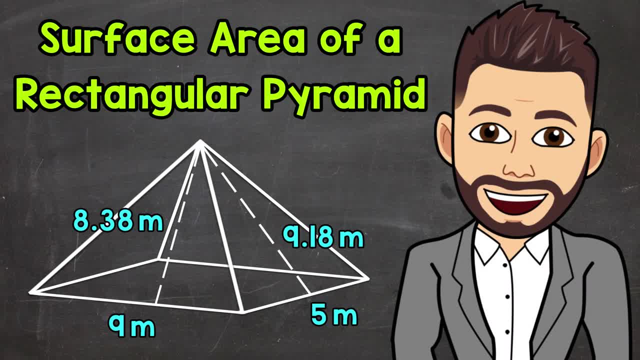 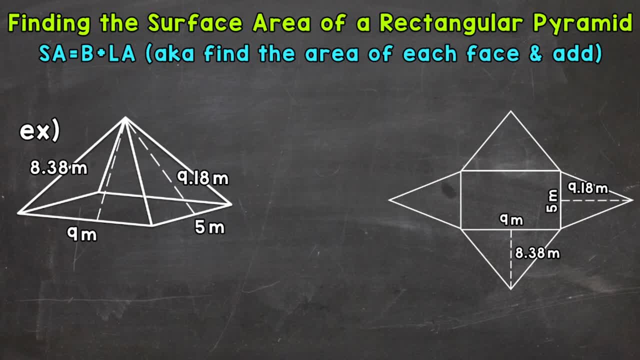 Welcome to Math with Mr J. In this video I'm going to cover how to find the surface area of a rectangular pyramid. And remember, surface area is the total area of the outside or surface of a three-dimensional shape. When it comes to rectangular pyramids, we have five total faces: the base and four lateral. 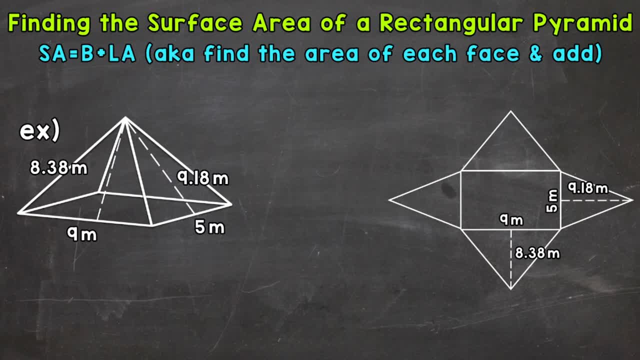 faces. The lateral faces are the triangular faces going around the pyramid, so to speak. We need to find the area of all of these and then add them together to get the total surface area. So let's jump into our example and start by writing out surface area. 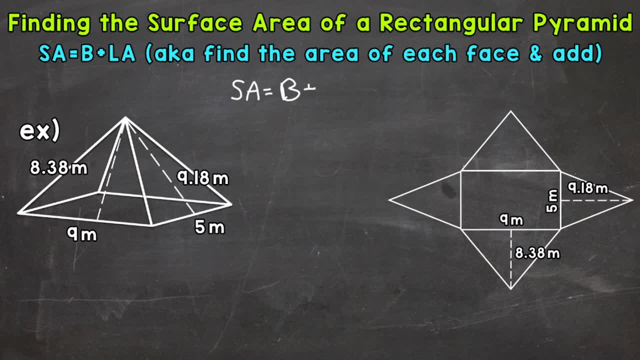 equals the area of the base plus the lateral area. Then we need to plug in our information, So we need to calculate the area of the base and all of the lateral faces, then add them together. Let's use the net on the right side of the screen to help us do this. You can think of a net as an. 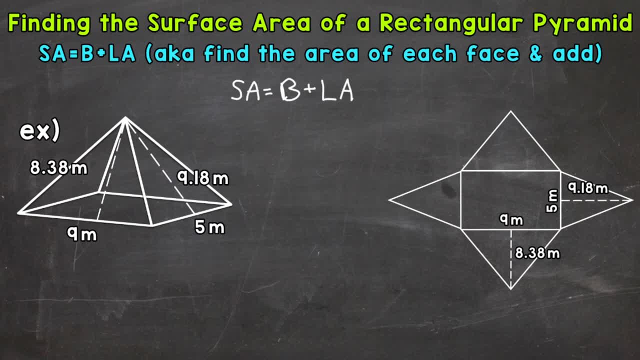 unfolded 3D shape. It shows us all of the parts, so to speak. Let's start with the area of the base. So we have a rectangular base, So we can use the formula area equals length times width. Now I'm going to use the formula area equals length times width. 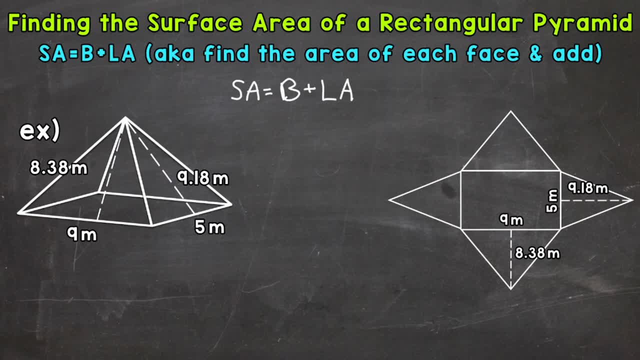 Now I'm going to use the bottom portion of the screen to show all my work as far as where I'm going to calculate the areas. So let's come to the bottom left area. equals length times width. Now we plug in, So our base has a length of 9 meters and a width of 5 meters, So 9 times 5.. Now if you use 5 for the 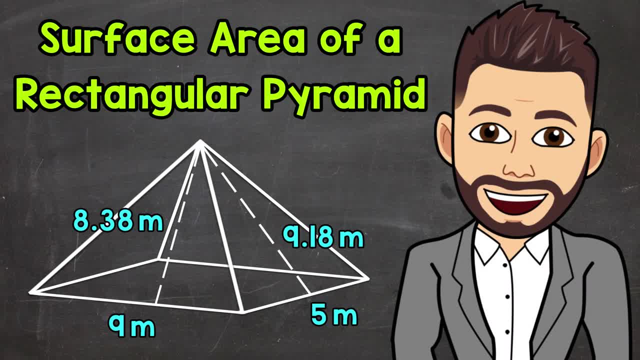 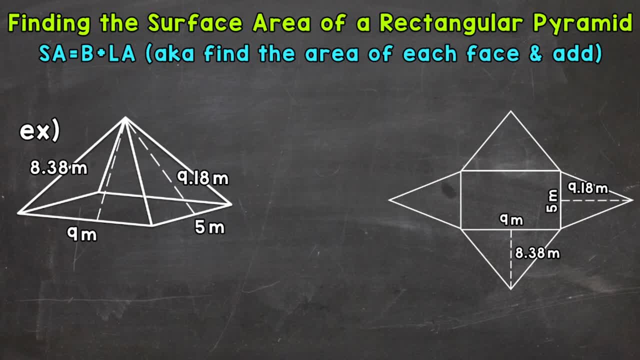 Welcome to Math with Mr J. In this video I'm going to cover how to find the surface area of a rectangular pyramid. And remember, surface area is the total area of the outside or surface of a three-dimensional shape. When it comes to rectangular pyramids, we have five total faces: the base and four lateral. 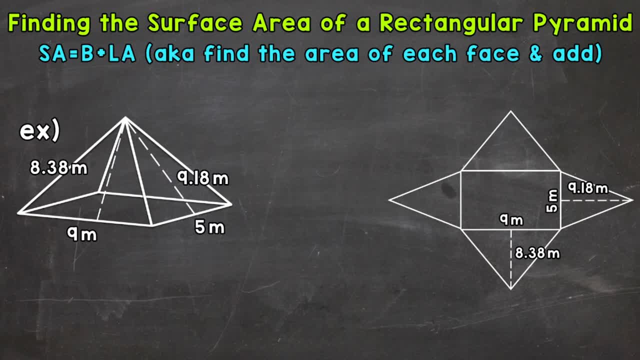 faces. The lateral faces are the triangular faces going around the pyramid, so to speak. We need to find the area of all of these and then add them together to get the total surface area. So let's jump into our example and start by writing out surface area. 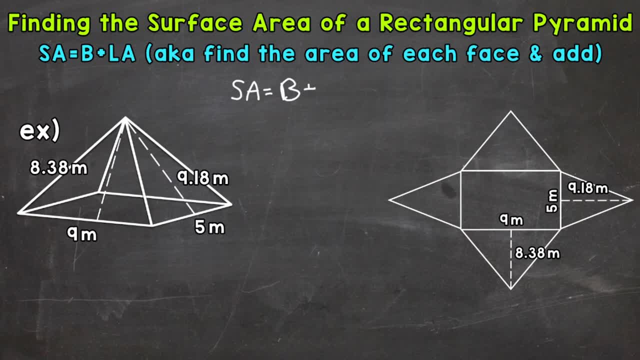 equals the area of the base plus the lateral area. Then we need to plug in our information, So we need to calculate the area of the base and all of the lateral faces, then add them together. Let's use the net on the right side of the screen to help us do this. 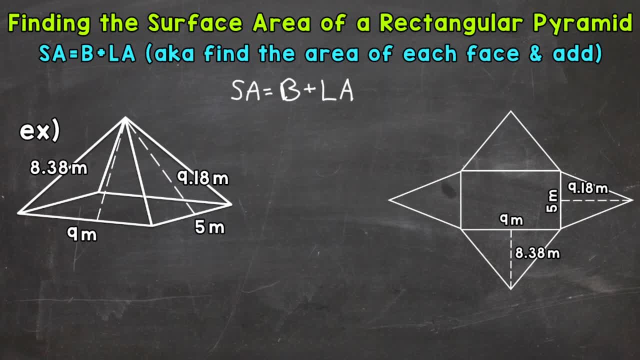 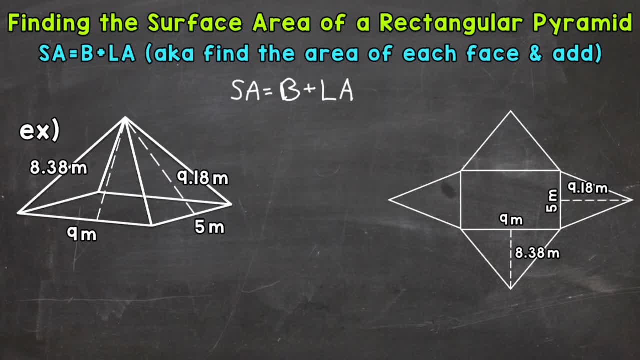 Now I'm going to use the formula area equals length times width. Now I'm going to use the formula area equals length times width. Now I'm going to use the formula area equals length times width. use the bottom portion of the screen to show all my work as far as where I'm. 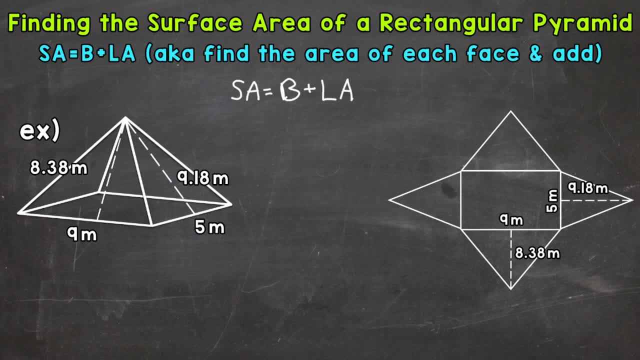 going to calculate the areas, so let's come to the bottom left area equals length times width. now we plug in, so our base has a length of 9 meters and a width of 5 meters, so 9 times 5. now, if you use 5 for the length and 9 for the 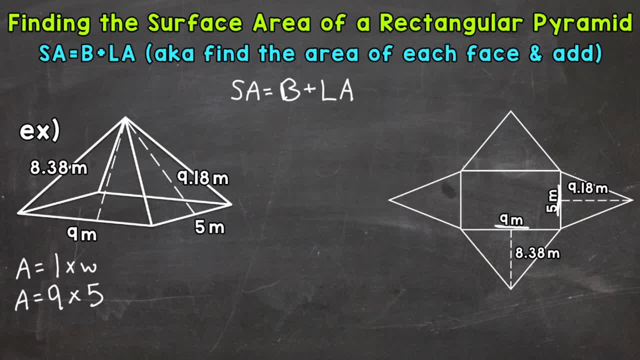 width, that would work as well. don't get too held up on which one is length or width, because 9 times 5 is the same as 5 times 9. both will give you the correct area. so the area of our rectangular base is 45 square meters. 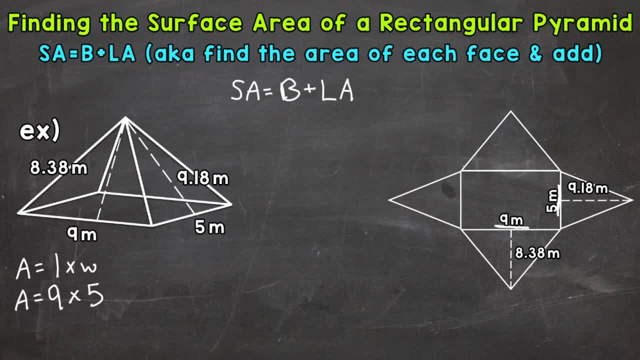 and 9 for the width. that would work as well. don't get too held up on which one is length or width, because 9 times 5 is the same as 5 times 9. both will give you the correct area. so the area of our rectangular base is 45 square meters. I'm 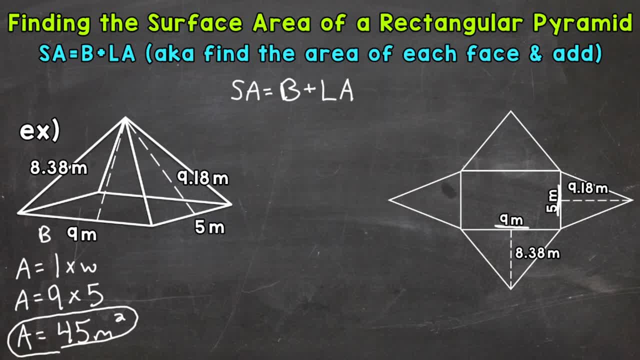 I'm going to put a capital B above that. so we know that that is the area of the base. now that we have the area of the base, we can move to the lateral faces. and since we do not have a regular base, regular means all of the sides are the 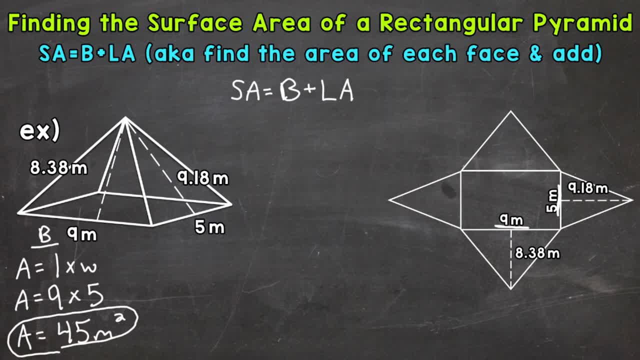 same, and this is not the case. this means that we will have two different slant heights and therefore two different areas for our lateral faces. these will have the same area and these will have the same area- the top and bottom of the net- because they have the same base- 9 meters- and same. 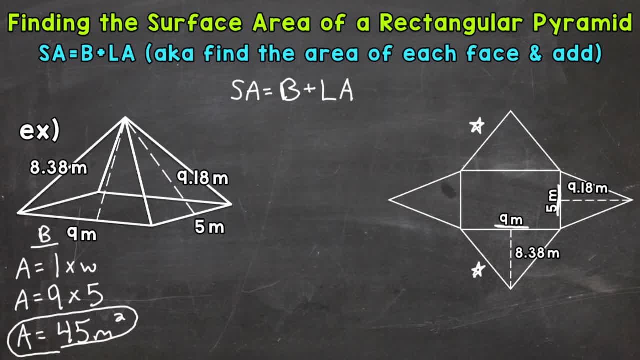 height, 8 and 38 hundredths meters. the left and right will have the same area because they have the same base of 5 meters and same height of 9 and 18 hundredths meters. so let's calculate the top and bottom lateral faces of the net. 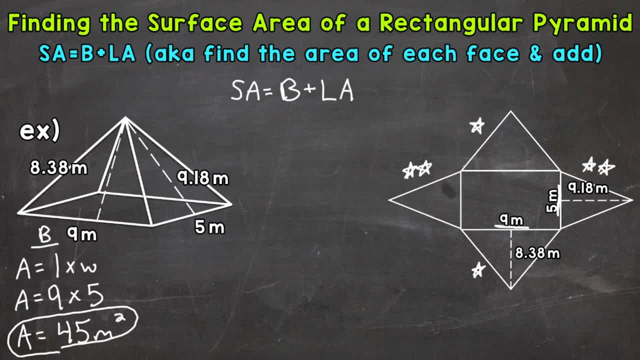 first, these would be the front and the back lateral faces of the 3d shape on the left hand side of the screen. now, since we're working with triangles, we can use the formula: area equals 1 half times the base times the height. so area equals 1 half times the base times the. 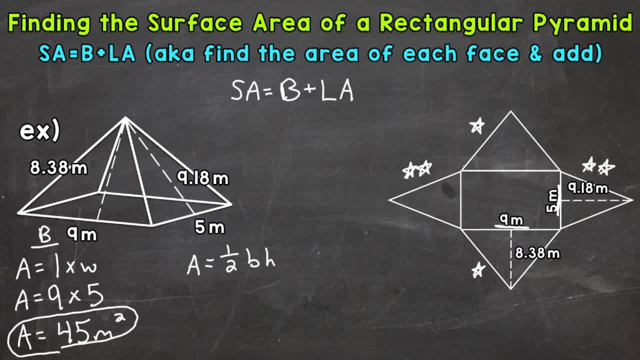 height. now you can also use base times- height divided by 2 for triangles, multiplying by a half or dividing by 2. they will get you the same answer. we're gonna do that now, So whatever formula works best for you, that's what you can use for finding the area of these. 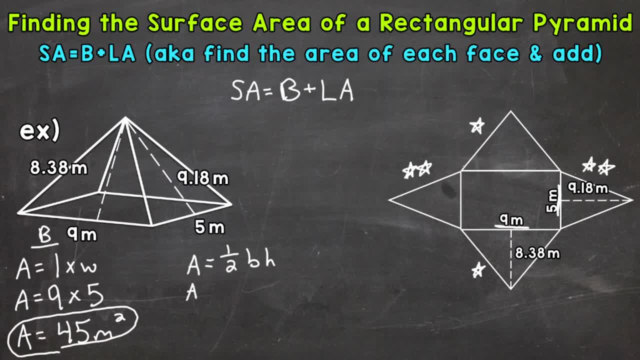 triangles. Now we plug in. So again, we're going to do the top and bottom from the net first. So 1 half times the base. Well, these have a base of 9 meters, So let's plug in 9 times the height. 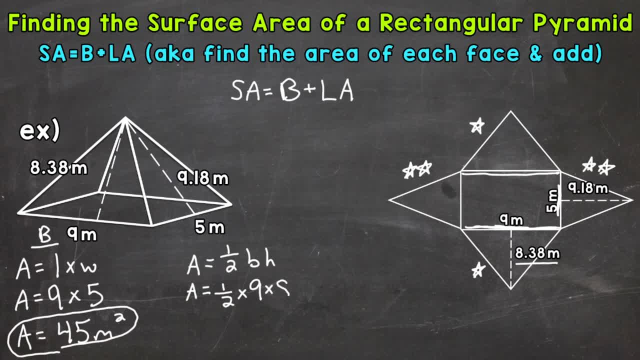 of 8 and 38 hundredths, And now we're ready to calculate. So the area of those lateral faces is going to be 37 and 71 hundredths, And this is square meters. Now I'm going to label this with one star above it, So we know that it is the top and bottom. 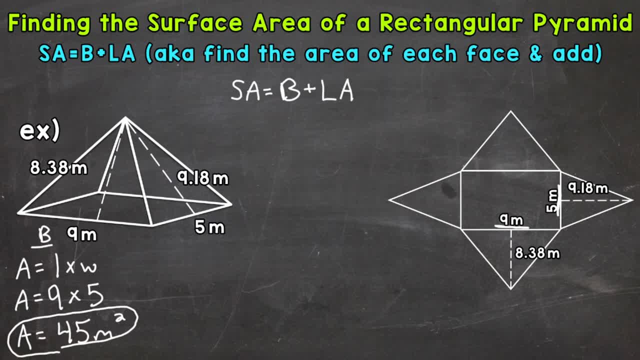 going to put a capital B above that. so we know that that is the area of the base. now that we have the area of the base, we can move to the lateral faces, and since we do not have a regular base, regular means all of the sides are the 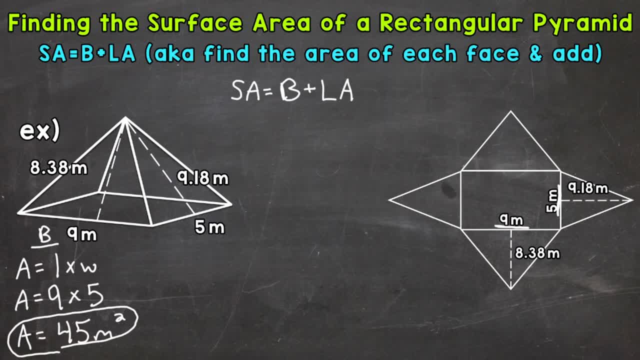 same, and this is not the case. this means that we will have two different slant heights and therefore two different areas for our lateral faces. these will have the same area- the top and bottom of the net- because they have the same base- 9 meters- and height- 8 and 38 hundredths meters. the left and right will have the same area. 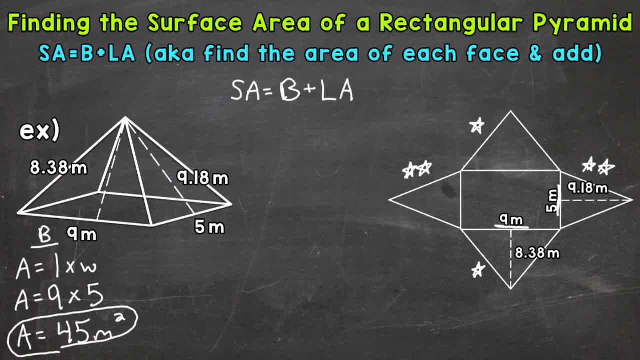 because they have the same base of 5 meters and same height of 9 and 18 hundredths meters. so let's calculate the top and bottom lateral faces of the net first. these would be the front and back lateral faces of the 3d shape on the. 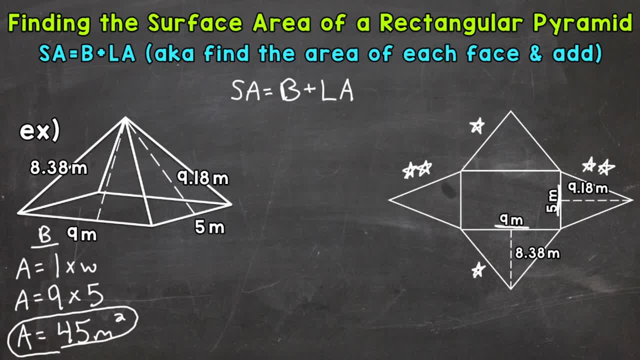 left hand side of the screen. now, since we're working with triangles, we can use the formula: area equals 1 half times the base times the height. so area equals 1 half times the base times the height. now you can also use base times height divided by 2 for triangles, multiplying by a half or 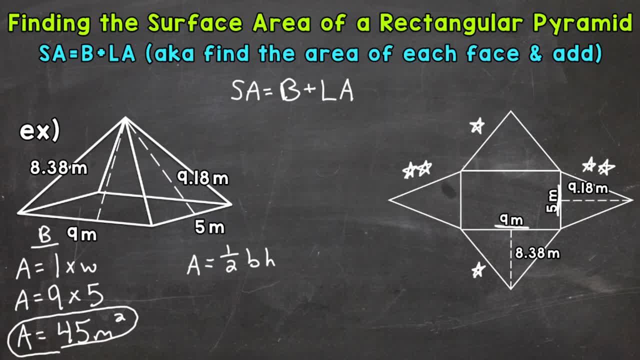 dividing by 2, they will get you the same answer. so, whatever formula works best for you, that's what you can use for finding the area of these triangles. and then now we plug in. so again, we're going to do the top and bottom from the net first. so 1 half times the base. well, these have a base of 9 meters, so let's. 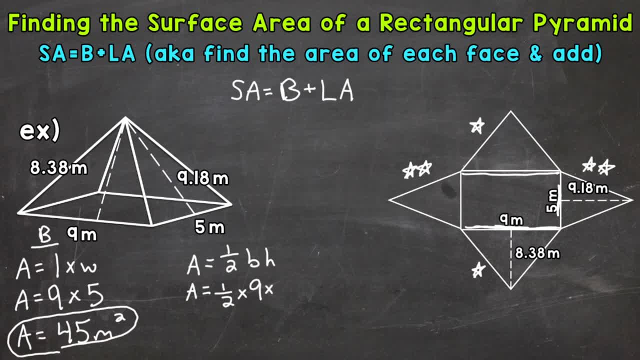 plug in 9 times the height of 8 and 38 hundredths, and now we're ready to calculate. so the area of those lateral faces is going to be an arch, and so now to be 37 and 71 hundredths, and this is square meters. now I'm going to label. 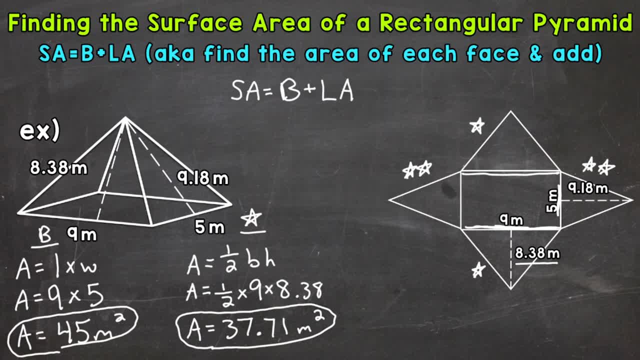 this with one star above it. so we know that it is the top and bottom lateral faces of that net. so we can move to the left and right lateral faces now and we have triangles. so we will write out our formula: area equals 1 half times base. 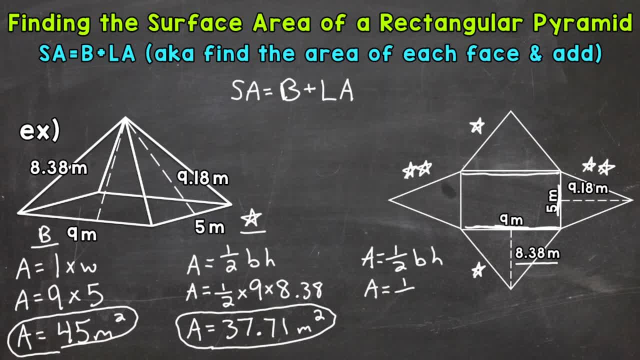 times height, and now we plug in, so 1 half, and these lateral faces have bases of 5 meters. so let's plug in 5 and a height of 9 and 18 hundredths meters. so 9 and 18 hundredths, now we calculate. so that's going to. 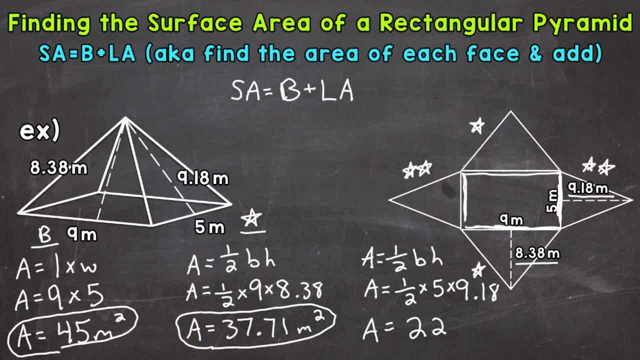 give us an area of 22 and 95 hundredths square meters, and I'm going to label this with two stars so we know which lateral faces have the area of 22 and 95 hundredths square meters. so once we have all of the areas calculated for our 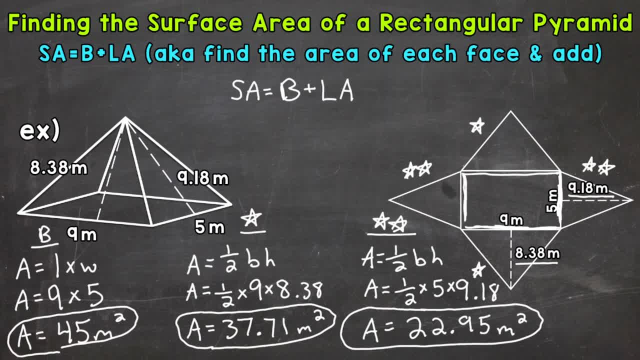 faces. we can fill in our net net to show exactly which areas go where, and it will help us stay organized. So we know that the area of the base was 45 square meters, So let's plug that in there. And then our one star lateral. 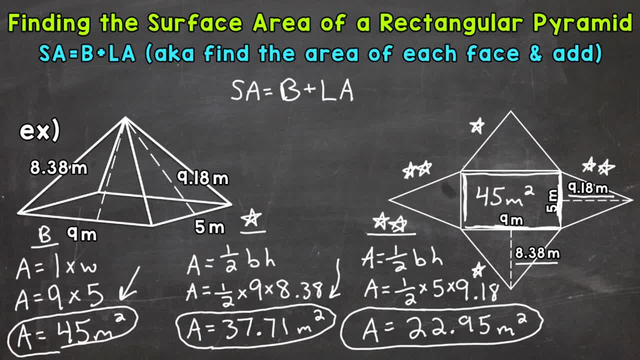 faces 37 and 70 one hundredths square meters. So let's label those And I'll put this one on the outside here. So 37 and 70, one hundredths square meters, And this goes right here. And now we have 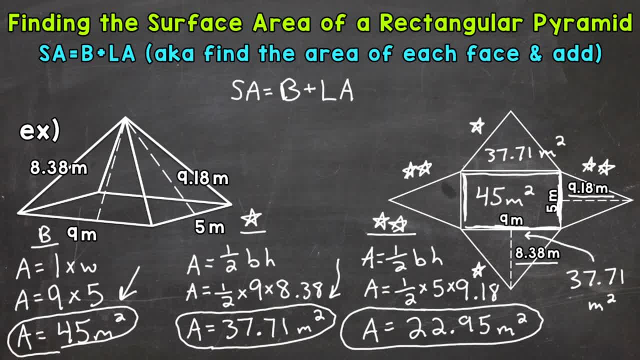 the two star lateral faces, the left and the right, 22 and 70.. 95 hundredths. So let's squeeze this in here: 22 and 95 hundredths square meters, And then 22 and 95 hundredths square meters goes right here, So we again have the areas for all of our faces, the base. 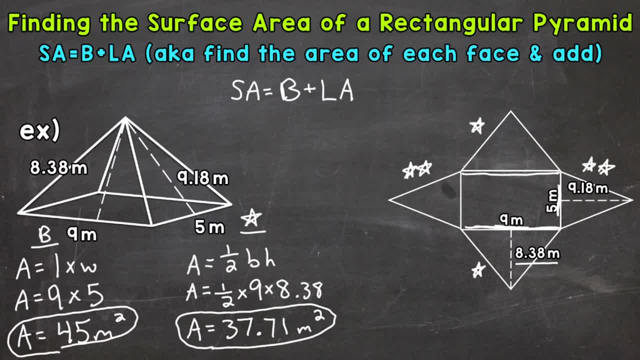 lateral faces. So we're going to do that, So we're going to do that, So we're going to do that of that net So we can move to the left and right lateral faces now, And we have triangles, So we 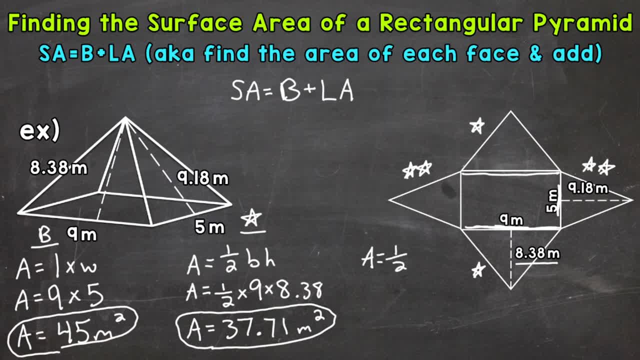 will write out our formula: Area equals 1 half times base times height, And now we plug in, So 1 half, And these lateral faces have bases of 5 meters, So let's plug in 5. And a height of 9. 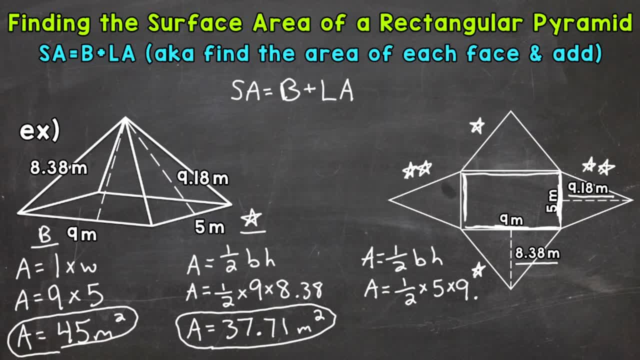 and 18 hundredths meters, So 9 and 18 hundredths- Now we calculate. So that's going to give us an area of 22 and 95 hundredths square meters And I'm going to label this with two stars So we know which lateral. 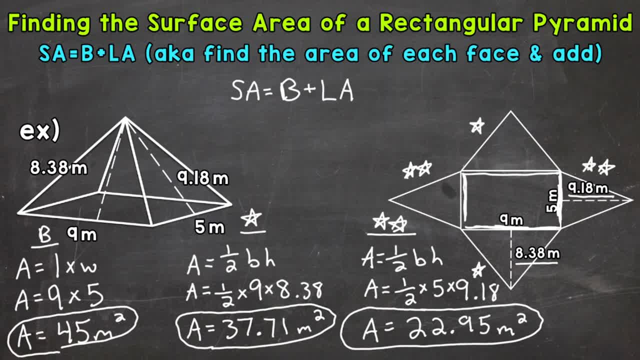 faces have the area of 22 and 95 hundredths square meters. So once we have all of the areas calculated for our faces, we can fill in our net to show exactly which areas go where And it will help us stay organized. So we know that the area of the base 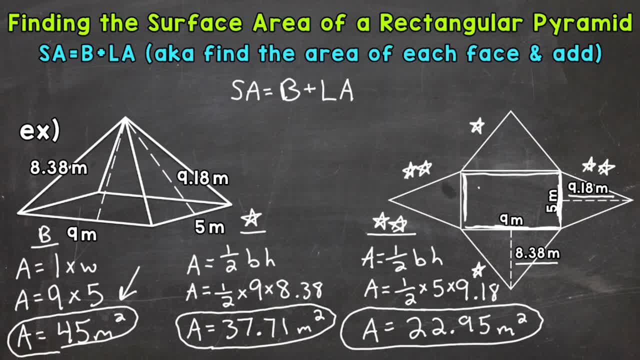 was 45 square meters, So let's plug that in there. And then our one star lateral faces 37 and 71 hundredths Square meters, So let's label those And I'll put this one on the outside here, So 37 and 71. 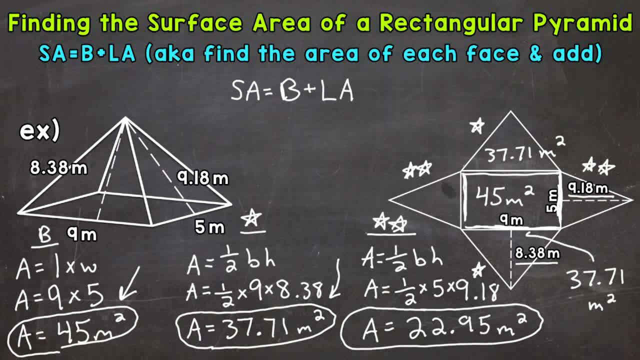 hundredths square meters, And this goes right here. And now we have the two star lateral faces, the left and the right: 22 and 95 hundredths. So let's squeeze this in here: 22 and 95 hundredths.